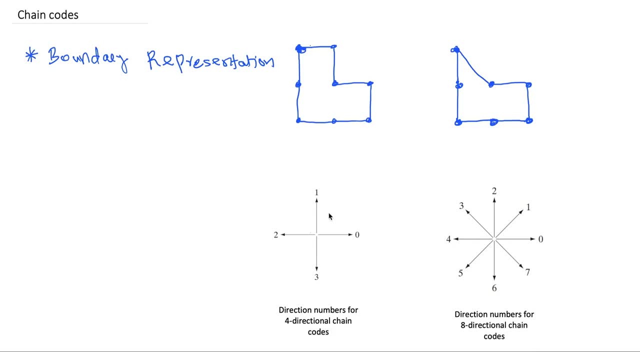 So the directional numbers of a four directional chain code is defined in this way. So if you have a straight line segment that is moving to the right side you have to use zero to represent that straightlin segment, and if the direction of the straight line segment is upward then we will be using number one to represent that segment. Then if it is to the left side then I will be using number two. If I have a straight line segment that is going down then I will be using number three to represent that straight line segment 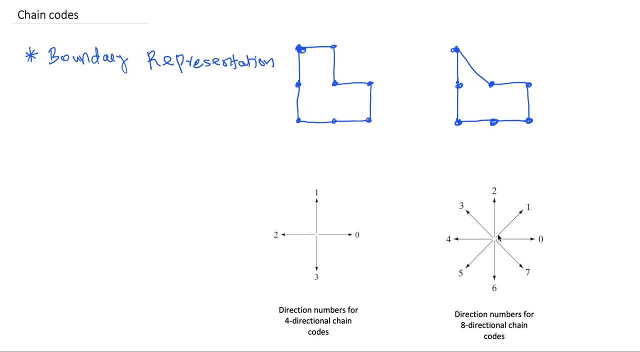 similarly the same kind of representation applies for a eight directional chain code also now we will look at how the chain codes can be created using these directional numbers to begin with we have to choose an initial point to start the coding from so by convention we will be choosing the top leftmost point so here this is the top leftmost point then you traverse in the clockwise direction okay clockwise direction now you take the first straight line segment from the starting point so have a straight line segment that is going to the right side so i'll be coding 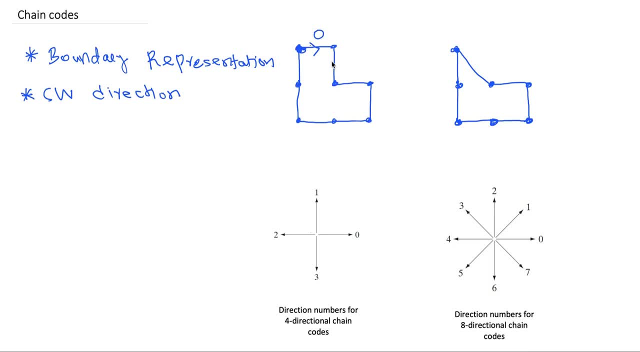 that segment with a number zero okay the next segment is going down so i'm writing the number three for that straight line segment because any downward direction has to be marked with number three the next segment is going right so i'll be again writing zero next one is downward so i'll be writing three next we have a segment that is 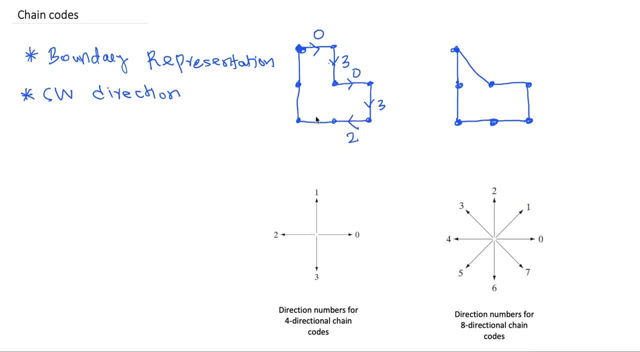 going to the left side so that has to be coded with number two again i have a straight line segment going to the left so again number two then i have a segment going up so i'll be coding it with 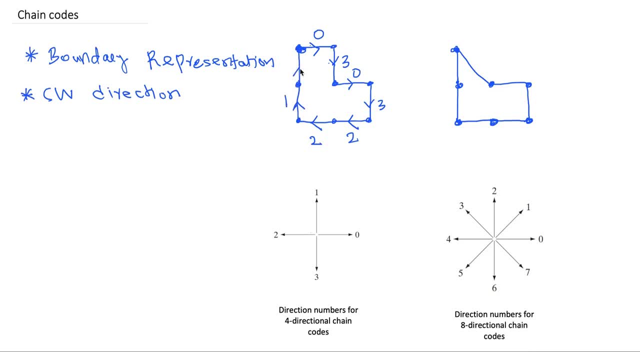 number one then again a segment that is going up i'll be numbering it with number one in order to write the chain code for this boundary you have to start from the starting point so the first code is 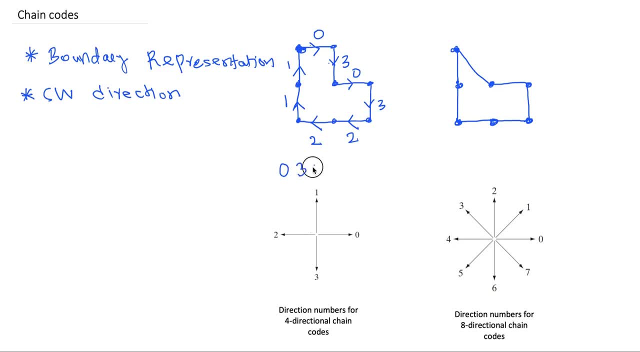 zero then you have three again zero again three then two two then one one okay so this is the chain 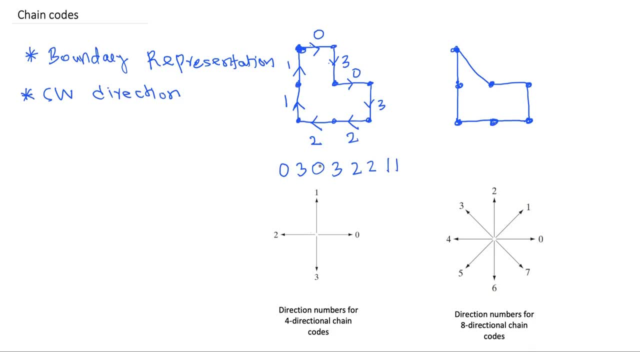 code for this particular boundary so this chain codes are also called freeman chain code now 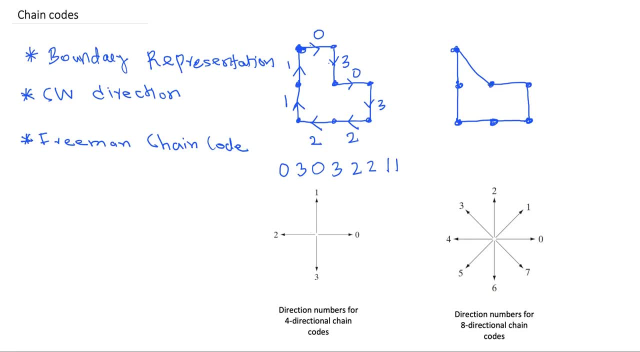 if you consider the second diagram we have a diagonal direction so we have to come up with a directional number for that segment also so we'll be using this convention if you have a 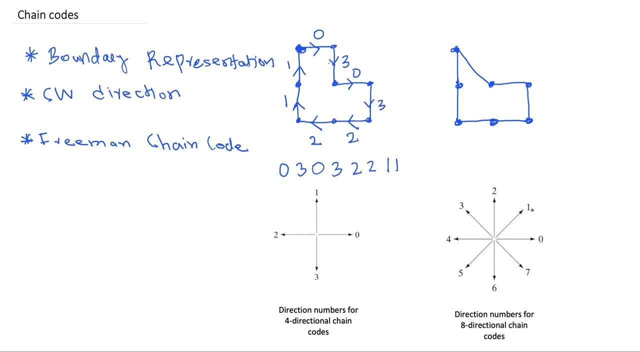 segment that is going diagonally up to the right side we'll be coding it with the number one 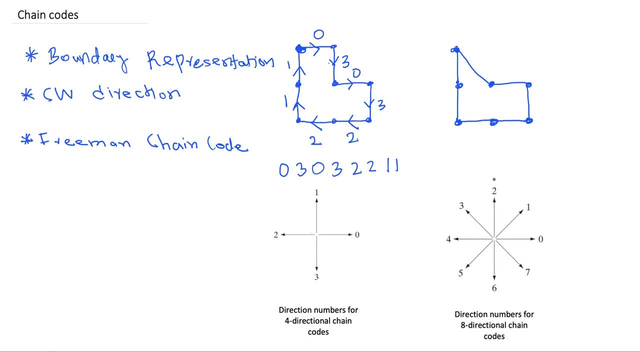 if you have a segment that is going up then we will be coding that with number two 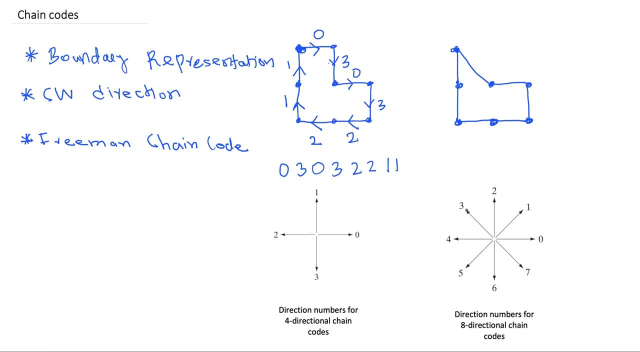 if you have a segment that is going diagonally up through the left side then you have to code it with number three and so on so we have to keep these two conventions in mind 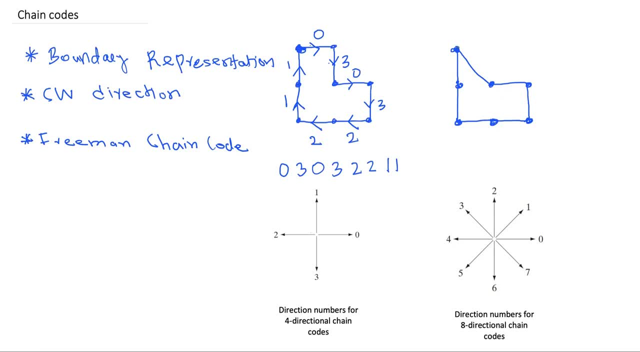 now we will code this particular boundary so we'll be starting from this point so the first number is the number corresponding to this segment so if you look at this image this direction is a 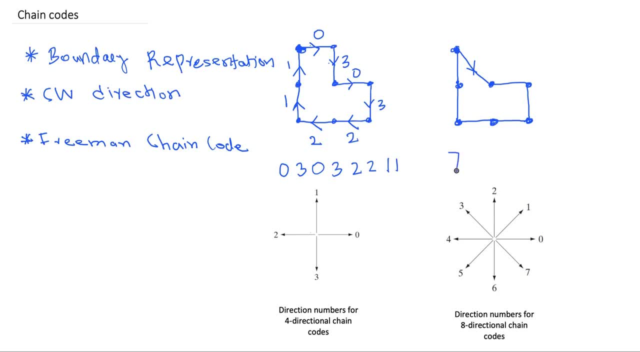 represented by using number seven so the first number will be number seven then you have a segment that is going to the right side so that has to be coded with number zero then one coming down so that has to be coded with number six 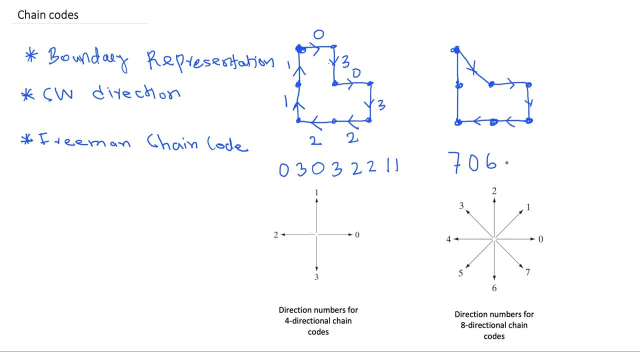 then we have two different lines going to the left side so that has to be coded with number four then you have two segments that is going up so that has to be coded with number 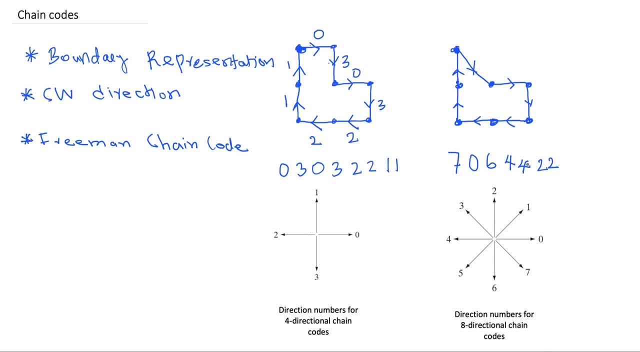 two okay so this is a Freeman chain code for the second boundary so this is number seven this is zero this is six this is four four then two and two okay 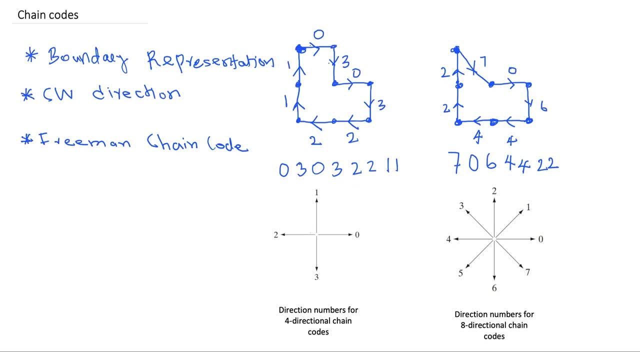 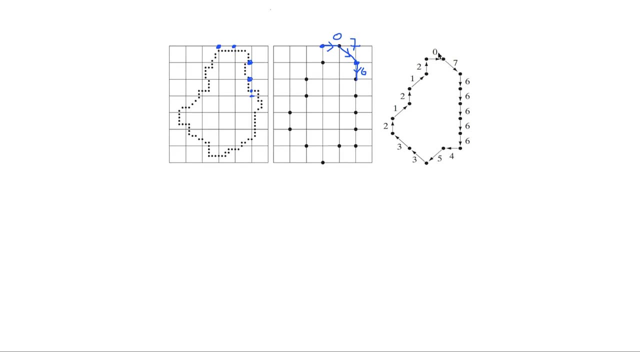 so this is how we form the Freeman chain code so finally you can come up with a chain code that is represented in this image and if you start writing the 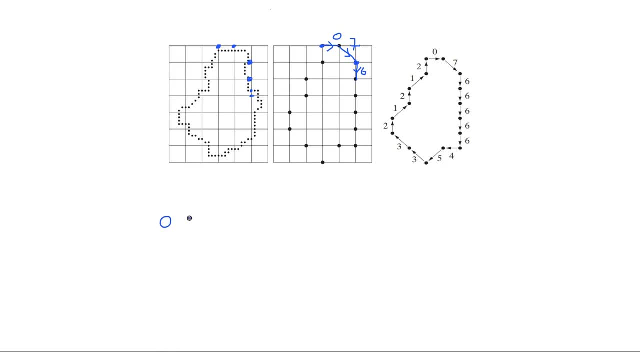 chain code from this point it will be zero seven six 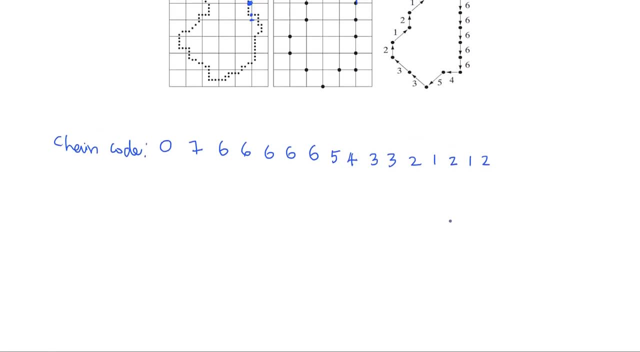 now suppose that I have a boundary as shown figure and now imagine that I am 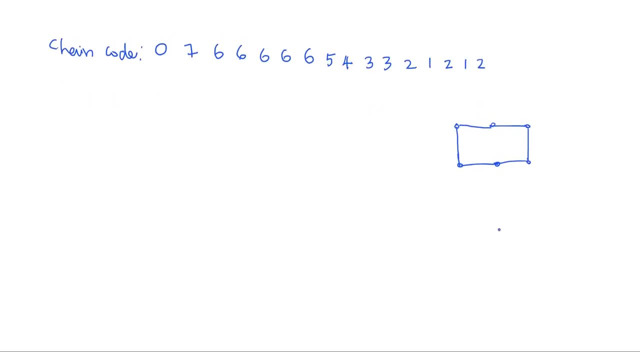 using the four directional chain code so we will have the directional numbers in this way so this is 0 1 2 & 3 now if I assign the directional code 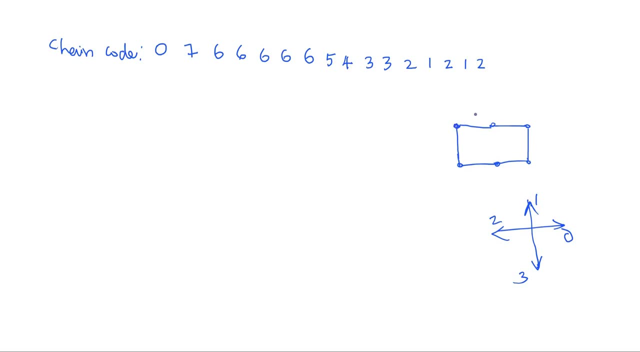 using these representation if I start from this point I will have 0 0 3 2 2 & 1 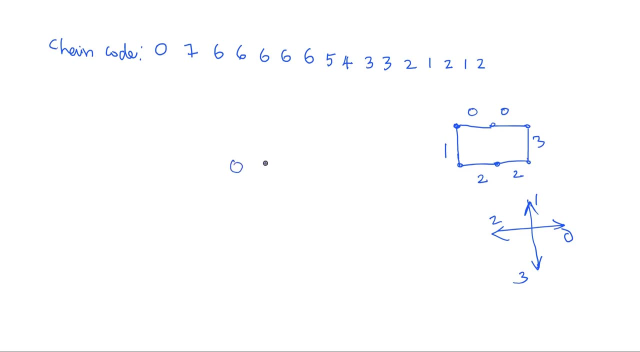 okay so the first chain code I have is 0 0 3 2 2 1 now what 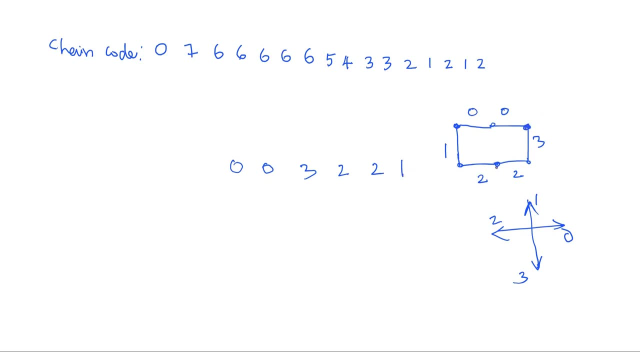 what will happen if I change my starting point to this point so the number will be 3 2 2 1 0 0 okay now what will happen if I have a starting point at this point 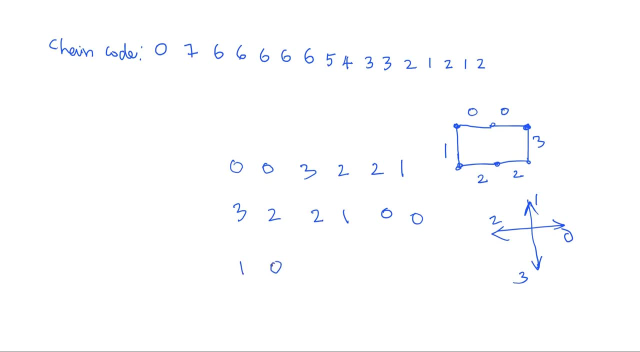 so that will be 1 0 0 3 2 2 so we have a problem here that is depending on the 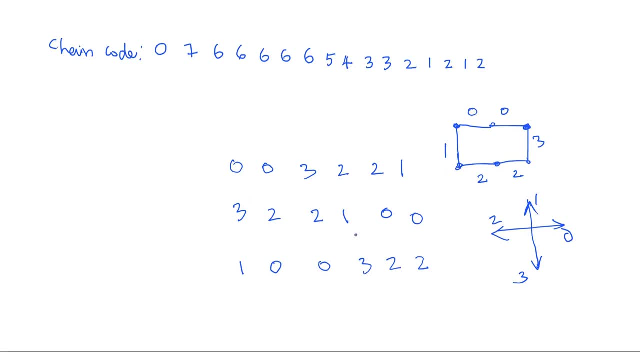 starting location of the chain code the code itself is varying so we have different Freeman chain codes for representing the same boundary okay so 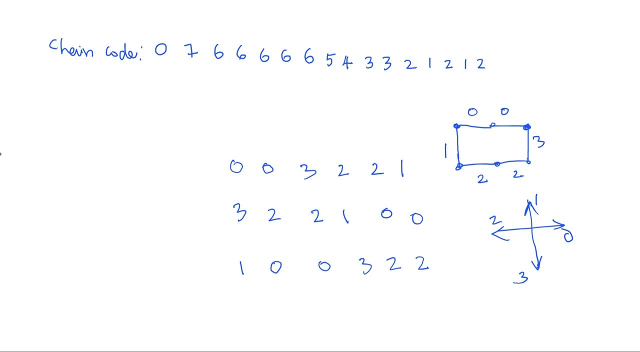 we have to resolve this problem in order to resolve that we have to normalize it with respect to the starting point okay okay in order to normalize these chain 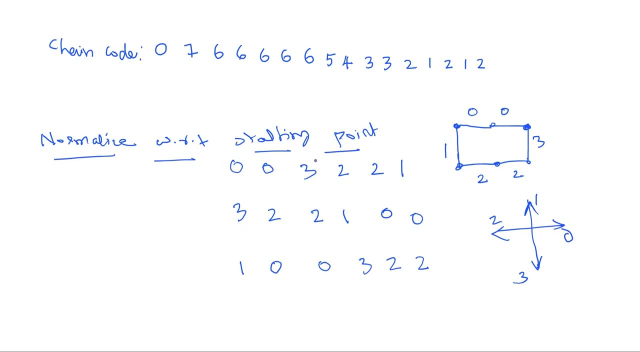 codes with respect to the starting point we have to treat this chain code as a circular sequence if you want to find the number after 1 then that number will be the number in the beginning so you have to just assume that we have written this number 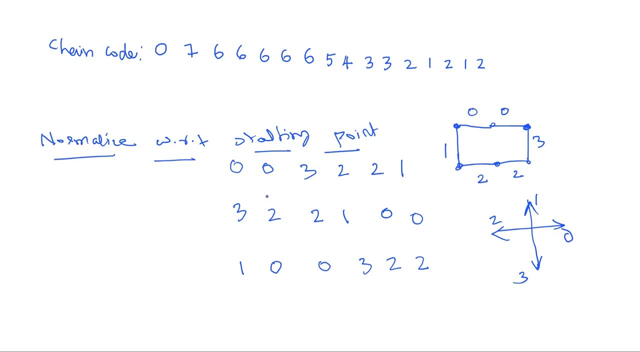 over the circumference of a circle we have to do one more thing that is we have to redefine the starting point such that the resulting integer has a lowest 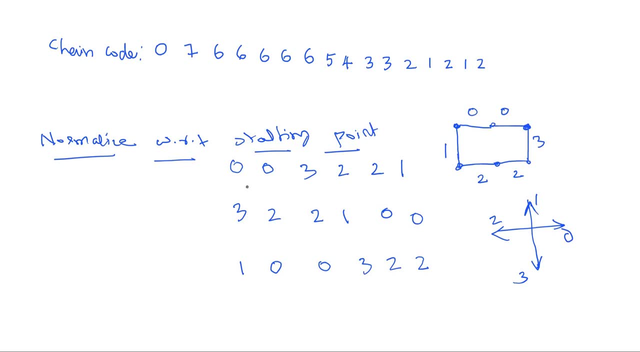 magnitude so for example if you treat this number as an integer this is actually three thousand two hundred and twenty one and if you treat this as an integer so this number will be three hundred and twenty two thousand one 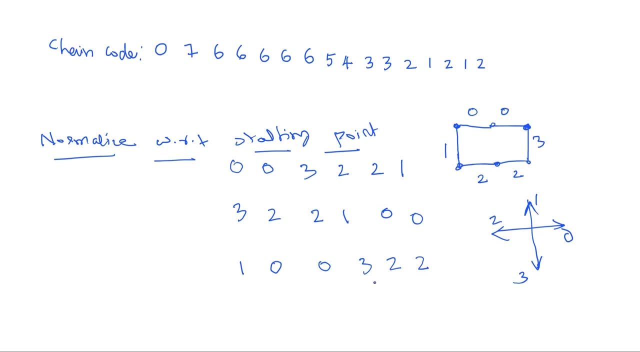 hundred okay so this will be a hundred thousand three hundred and twenty two okay so whichever number gives a smaller magnitude we have to take that number as the chain code so in 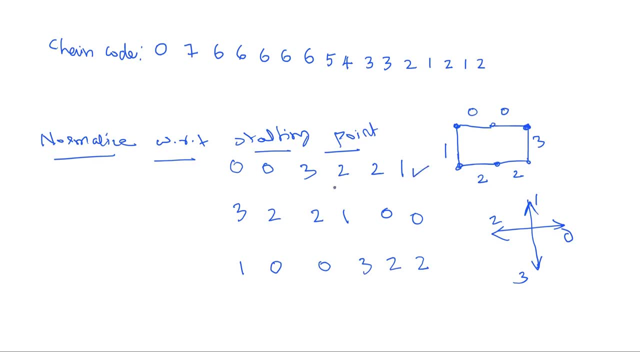 these three options we will have to choose this one because this has the lowest magnitude if you want to get a simple example suppose that I have a 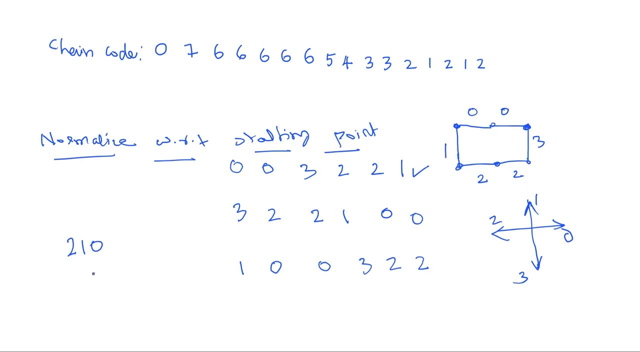 number 210 if I rearrange this number one option will be 0 21 and another option will be 102 okay so these are different options that 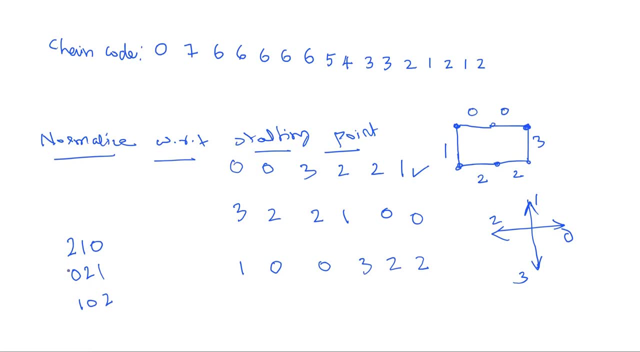 I can come up with by changing the starting point assuming that these numbers are behaving circularly this is 210 this is 21 and this is 102 sort of 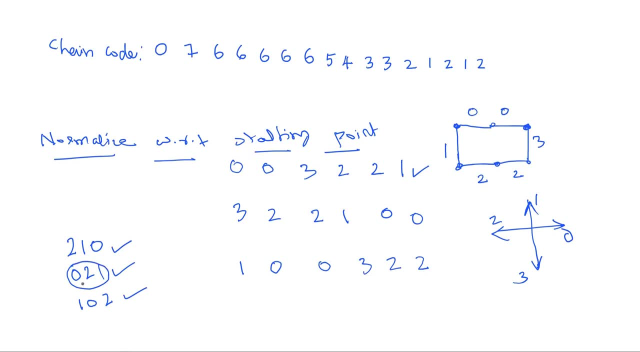 this I need to select this number because this is the number 21 and which 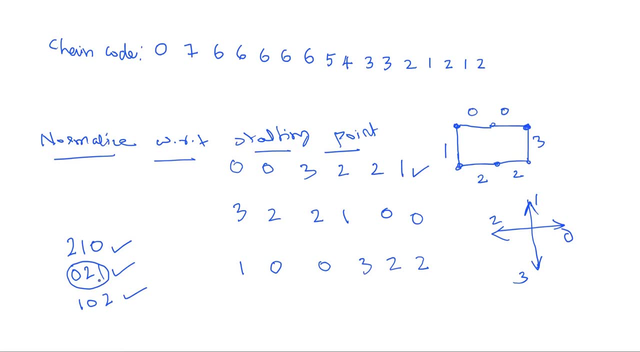 has the lowest magnitude among these three numbers okay so in order to normalize with respect to starting point we have to so in order to normalize it with respect to starting point I have to select the starting points such that 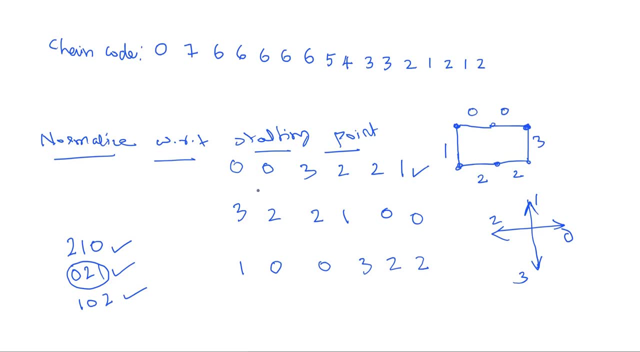 the resulting chain code gives the lowest magnitude okay so among these three I will be selecting this one now as a result of normalization with 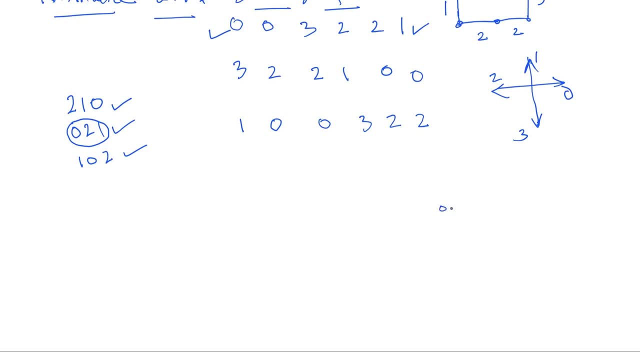 respect to starting point imagine that I have a boundary of this kind okay now if 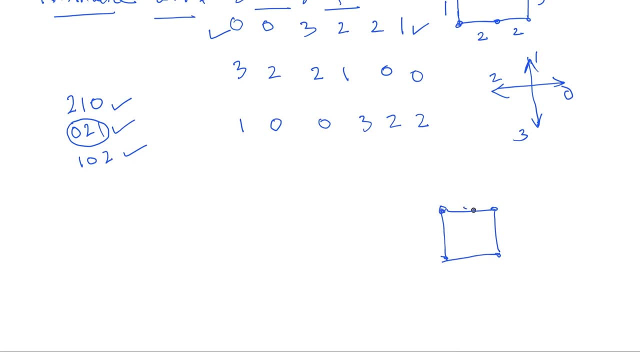 I choose to start from this point then the chain code will be 0 then 3 then 2 then 1 okay so I am writing the chain code that is zero three two one and if I 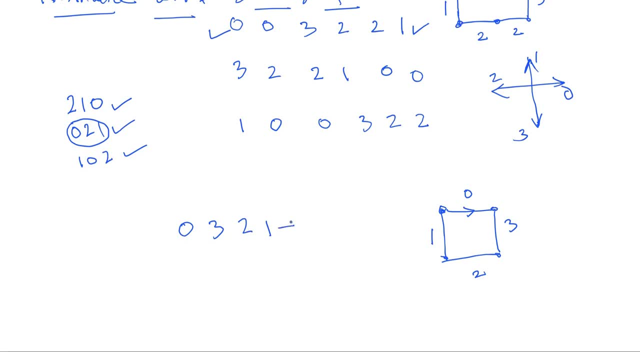 assume this number as a circular sequence and if I want to get the smallest magnitude number from this one then it will be the same number that is 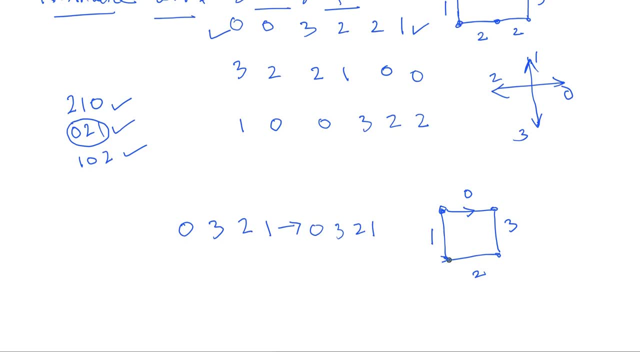 zero three two one and if someone decide to start from this point then the 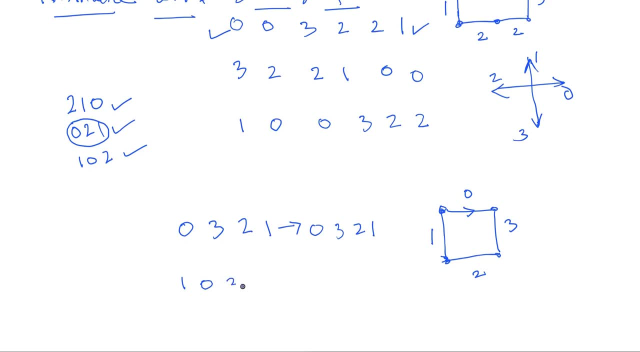 corresponding chain code will be one zero three two then we will have to rearrange this number such that we should get the smallest 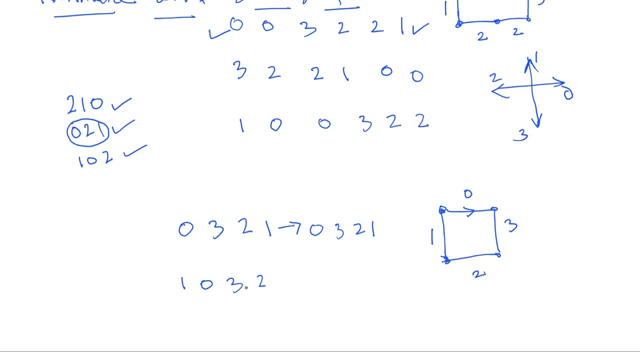 two number so in order to normalize this number you have to come up with the smallest magnitude number so it will be by taking the number zero in the beginning so we'll get 0 3 2 1 so those 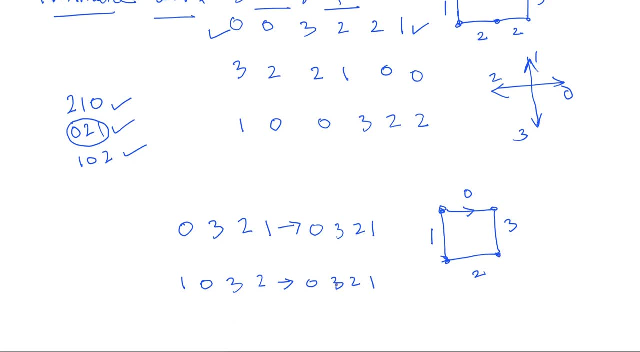 two numbers are again the same and if someone decide to start from this point then the number will be 2 1 0 3 and if you normalize this number again then you have to bring the zero to the 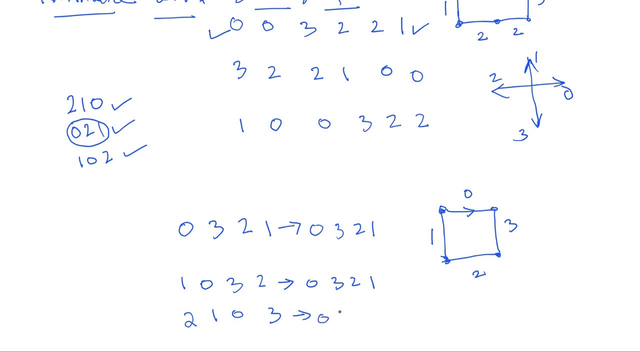 beginning then only we will get the smallest magnitude so the resulting number will be 0 3 2 1 so it doesn't matter where you start once you normalize with respect to the starting point 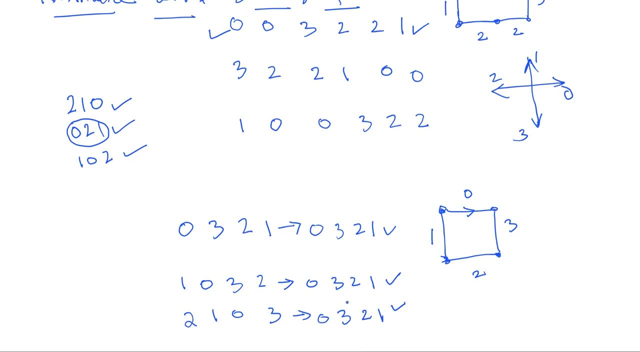 the chain code will not differ it will be the same now we have to tackle one more issue in the chain code imagine that I have two different boundaries over here 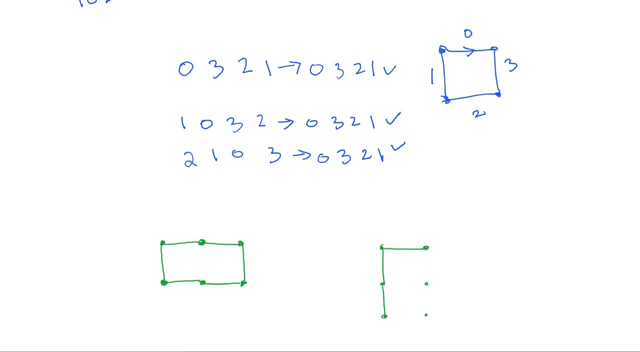 when you look at the first image and the second image the second image is the rotator version of the first image if you try to find the chain codes of these two boundaries using the directional 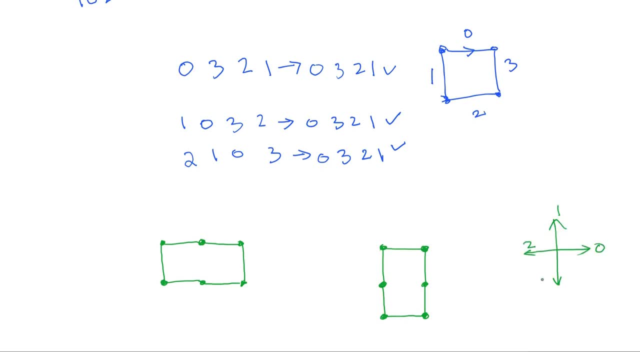 codes like this one then it will be as follows here I am taking this as the starting point then the first code will be zero then again 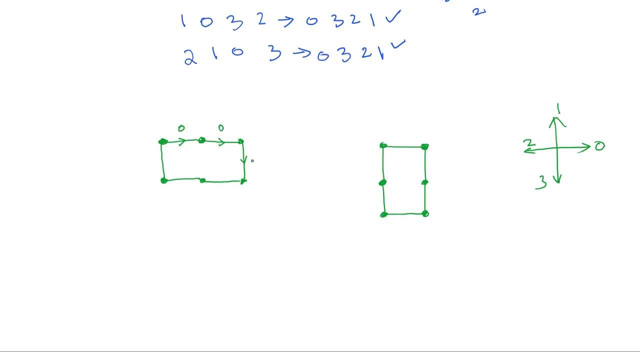 zero then we have the next code as three then two again two then we have the last number as one so 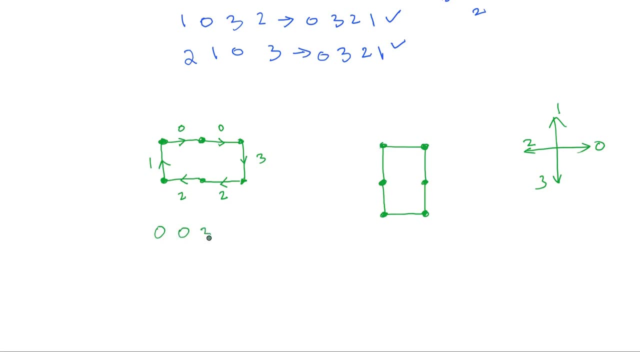 the chain code is 0 0 3 2 2 1 okay now we don't want to normalize it because it has the smallest 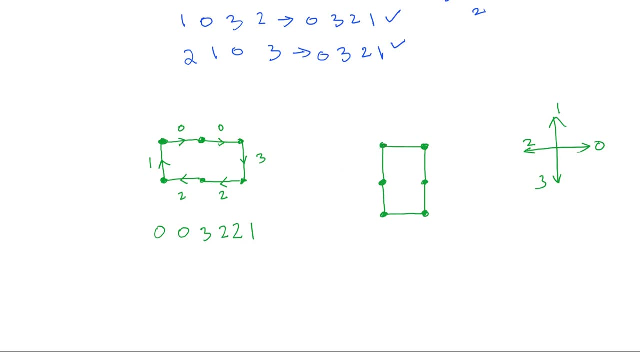 magnitude itself now if you look at the second one if I take this one as the starting point 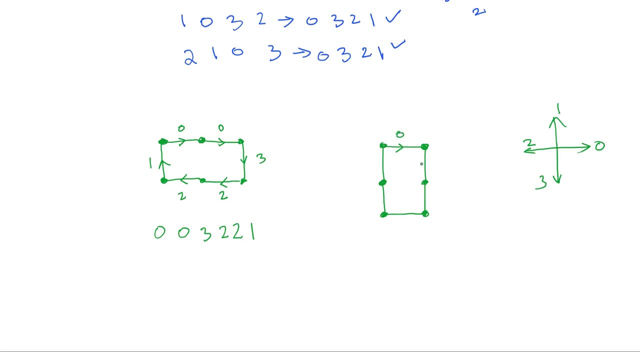 it will be 0 0 3 2 1 and if you look at the second one if I take this one as the starting point it then the first code will be zero then i have three again three then two then one and again one okay 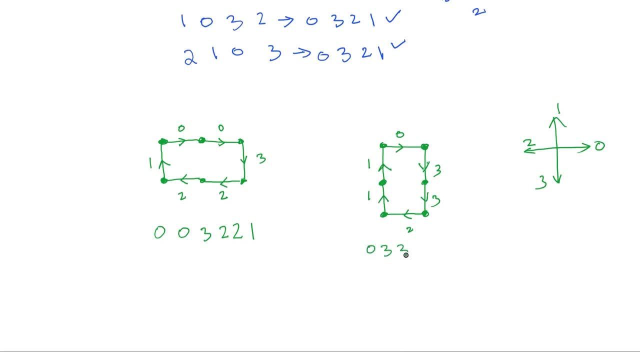 so the chain code will be zero three three two one one okay so when you look at these two codes these two codes are completely different even if i consider it is a circular sequence it will not be the same sequence at all when you look at the boundaries one is the rotated version of the other one if you show a boundary of this kind to the computer first it will calculate its chain code as follows and if you rotate the image and again show that boundary to the computer then this will be the chain code the computer will determine that these two images are completely different but actually they are the same but the difference is one is a rotated version of the other one 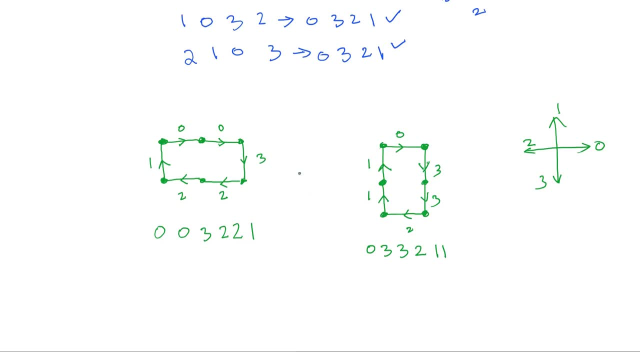 then how can we tackle this issue that is even though one image is a rotated version of the other one i need to get the same code for both the boundaries okay so for this purpose we have to normalize the chain code for rotation in order to normalize the chain code for rotation rather than writing the chain code as itself we will write the first difference code of the chain code the first difference of the chain code is obtained by writing the number of direction changes that separates two adjacent codes in the first chain code so this is my chain code by the first difference code 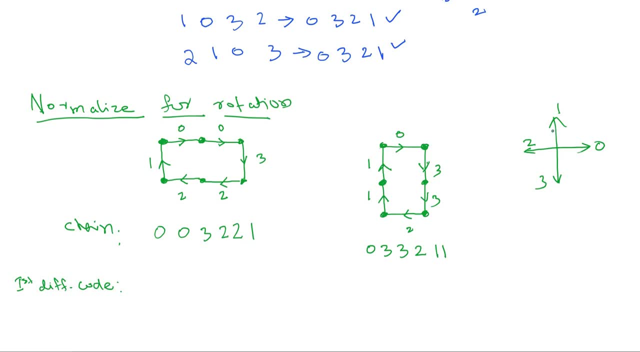 okay so here you have the direction one as we are treating the chain code as a circular sequence in order to get the first element of the difference code we have to count the number of direction changes it takes from 1 to 0 if you are moving this directions and the clockwise direction 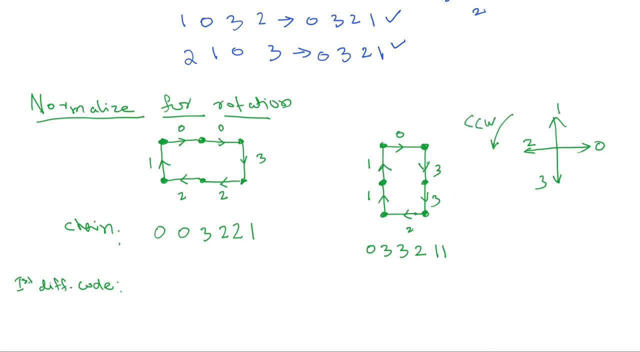 okay so we are moving in the counterclockwise direction starting from direction 1 we will be counting the number of directional changes it takes to reach the direction 0 so there is one direction change when it comes from 1 to 2 and another for 2 to 3 and another 4 3 to 0 okay so the first element of our difference code will be 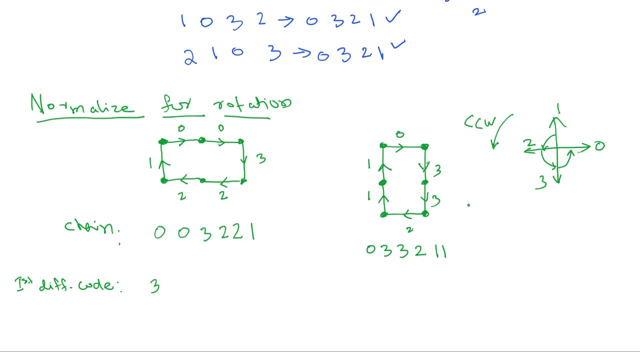 3 because we have taken three different direction changes to reach from 0 to 0 i do not need any direction changes so the number of direction changes is 0 so that comes as the second element of my difference code then from 0 to 3 then this is 0 then to reach 3 i need to take 1 2 3 3 direction changes so the next element of my difference code is 3 then from 3 to 2 if you count it then i have this is 3 to reach 2 i need to take 1 2 3 so again 3 okay then from 2 to 2 i